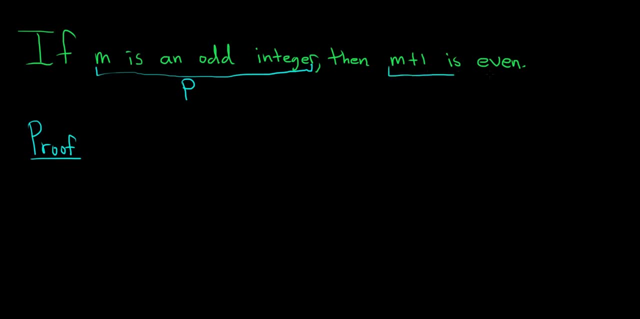 then q type statement, And so in order to give what's called a direct proof. so the normal, usual way of proving this is: you assume that p is true, So you assume p, And then, via some steps, you show that q is true, And once you've done that, you've proven it. so it's. 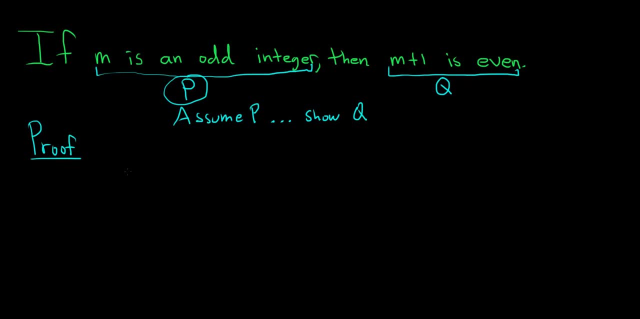 always true, no matter what It is considered an absolute truth in mathematics. So let's start our proof by writing down our assumption, which is p. So you start by saying: suppose that, And then I'll just take it verbatim from the question that m is: 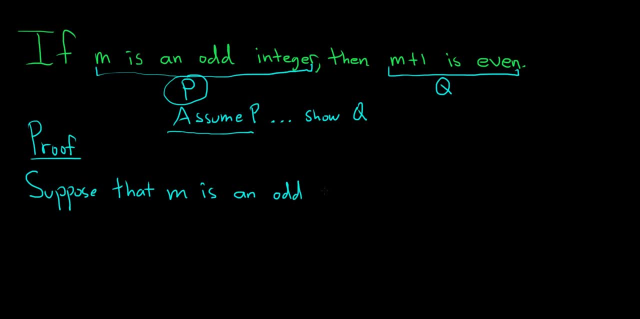 an odd integer. Now, immediately the mind jumps to q. It could be because you have to show q is true. m plus 1 is even. However, you can't do that right away. In order for the proof to work, you have to use your hypothesis, In other words: 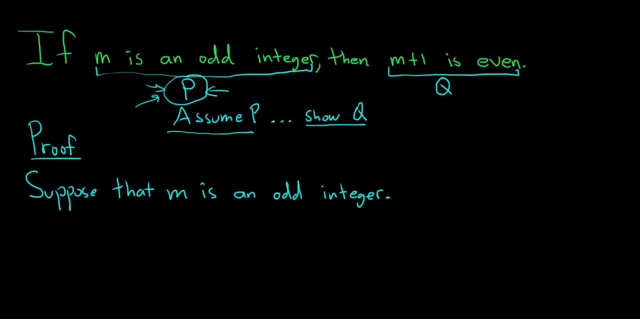 you have to use the truth of p to show that q is true. So typically what you do in these types of proofs is you just write down what it means. So you have something written down on the screen and you say, hey, what does that mean? 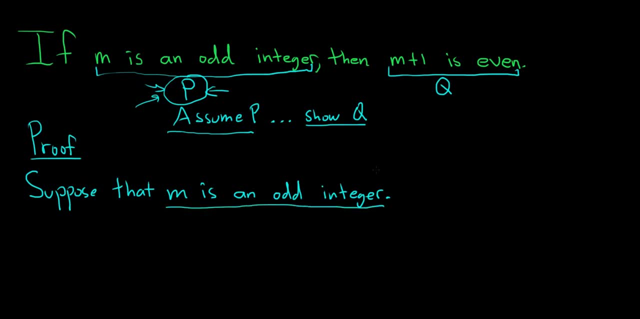 What does it mean for m to be an odd integer? So this is where you have to know the definitions. So there's two definitions in this problem that we'll need. The first one is for an odd integer. So we say that b is odd. 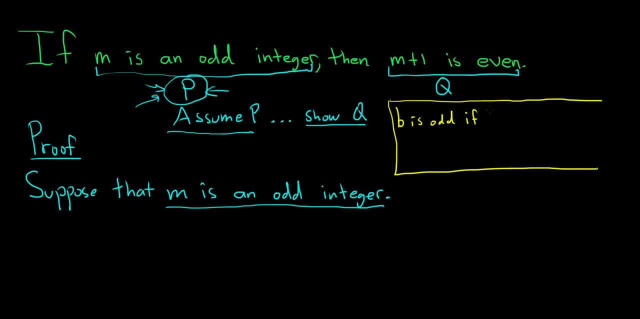 if you can write b as 2 times an integer plus 1.. So I'll go ahead and use the variable k for our integer. So b equals 2k plus 1, where k is an integer And we'll say b is even. 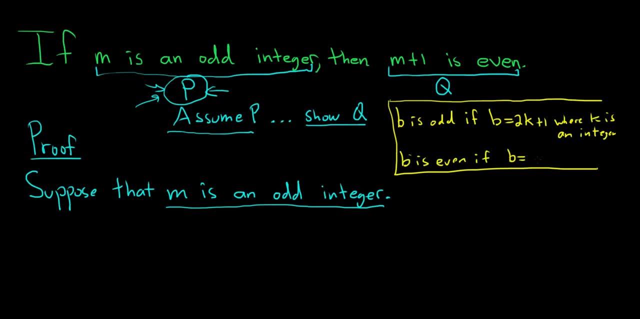 if? well, it's very similar. If b is equal to 2, and we'll say b is even. if b is equal to 2,, then I'll use a different letter this time: 2n, where n is an integer. 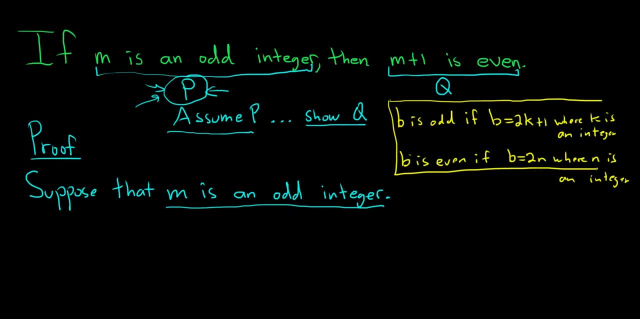 So definitions and proofs are absolutely vital. Like without the definitions, it often you won't be able to do it. Most of the time when people get stuck in proofs is because they don't understand the structure or they don't really know the definition. 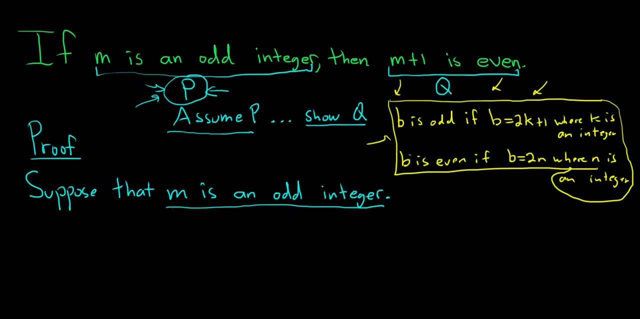 So if you have those two things, you'll make it very far. So in this case, m is an odd integer, so let's write down what that means. So this means that m is equal to- I'll use the same letter- 2k plus 1,. 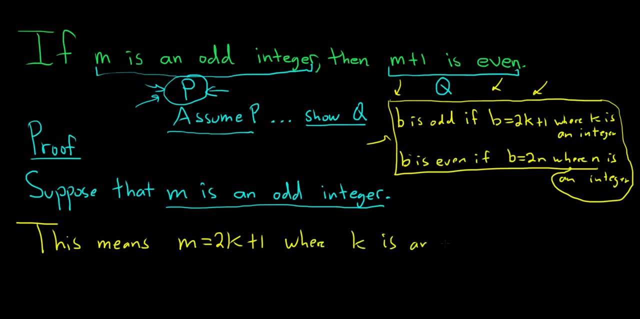 where k is an integer. So at this point we've pretty much exhausted our hypothesis. You know, we wrote down our assumption and we wrote down what it meant, And so now we have to look at q and we're trying again to show the validity of. 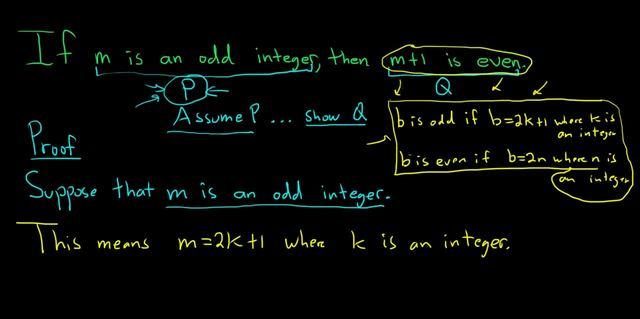 of q. So the natural thing to do is to write down m plus 1 and try to figure out what that is. So then, m plus 1, well, m is equal to 2k plus 1.. So 2k plus 1,. 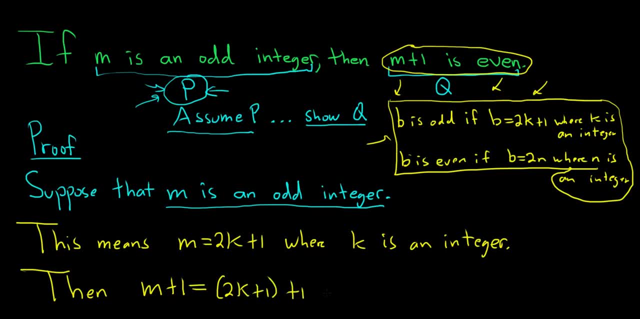 and then we still have a plus 1 hanging out here. And here's where the magic happens: 1 plus 1 is equal to 2, right? That's the key step, or not quite. We can factor something out now. 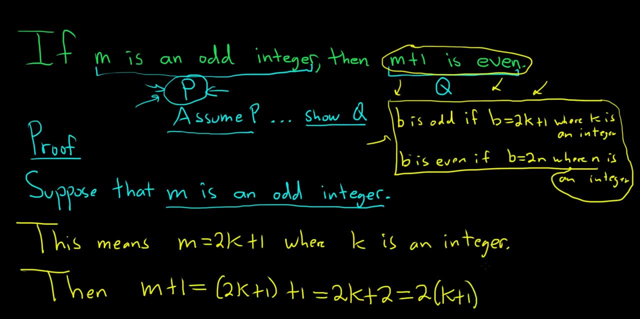 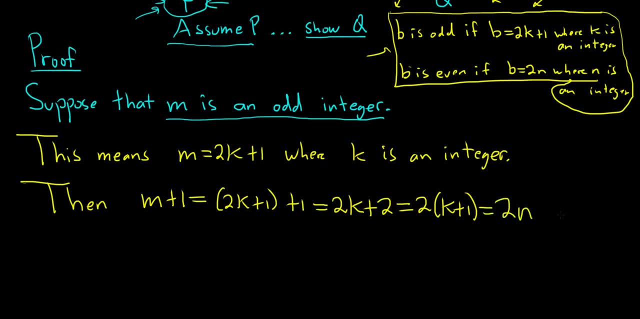 You can pull out a, 2. So you get 2 times, 2 times k plus 1.. And here's where we're going to do a little cool move, which is equal to 2n And say what's n. 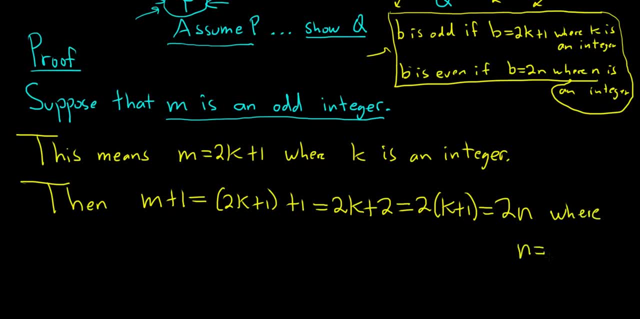 Well, we made it up where n equals k plus 1 is an integer. So we showed that m plus 1 is equal to 2 times an integer. So that's exactly what it means for m plus 1 to be equal to 2 times an integer. 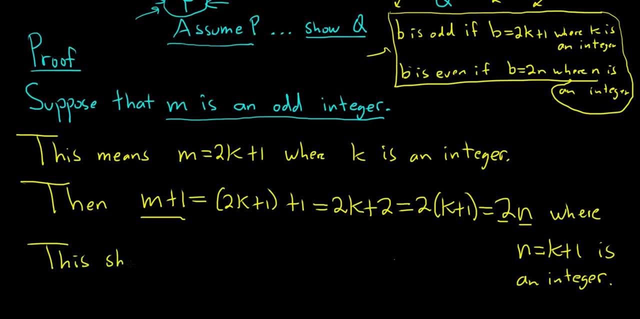 So this means, or this shows, m plus 1 is even And the proof is complete, And so I'll use a little box with an x. The old way of doing it is qed. The modern way of doing it, to finish the proofs, is a filled. 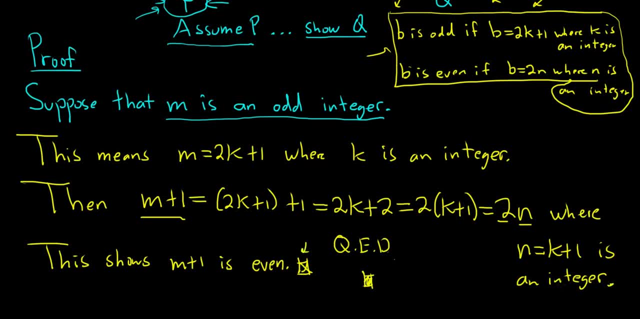 in box. I use a box with an x, So that completes the proof. And you might be wondering: why is k plus 1 an integer? Well, if you have an integer plus an integer, you always get an integer, So let's call it an integer.